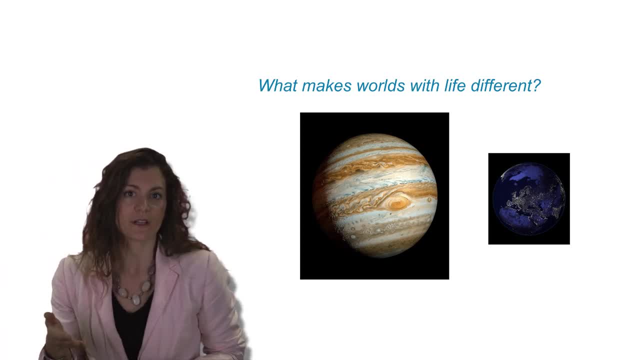 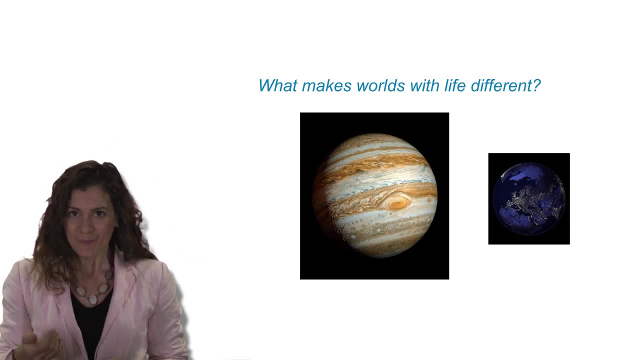 it's clear that both have nonequilibrium structures on their surfaces. So Jupiter, for example, has a habit of coincidence. When we look at Europe, for example, you have a habit of coincidence: has this great red spot And, as I mentioned, Earth has cities. So when we want to talk about 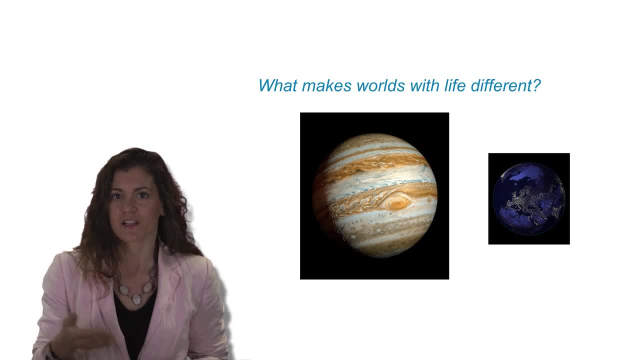 defining the properties of those planets that are associated with life. it's not just about this disequilibria. Clearly, cities are fundamentally different than the great red spot of Jupiter, even though they're both non-equilibrium structures. So we have to move. 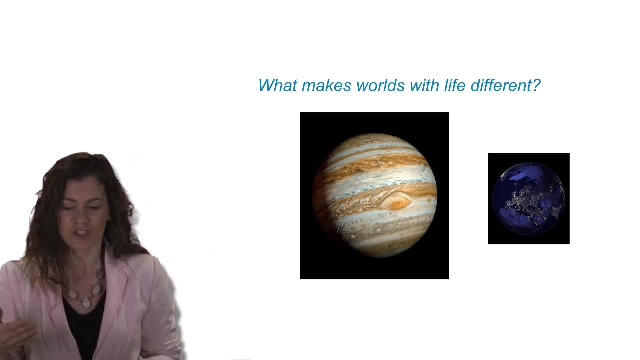 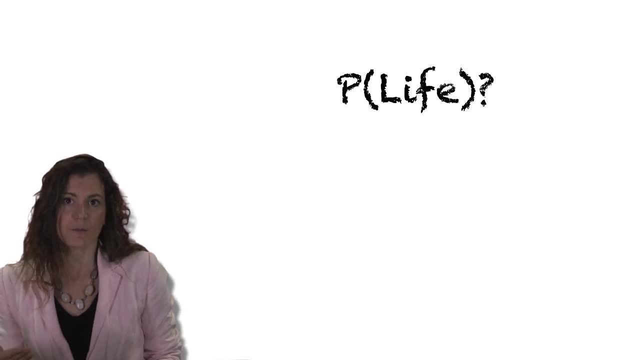 a little bit further and understand the origins of the processes that led to structures on the surface of our planet that are associated with life. And the root of that question is really to understand what's the probability of life emerging on a planet, and how can we actually understand? 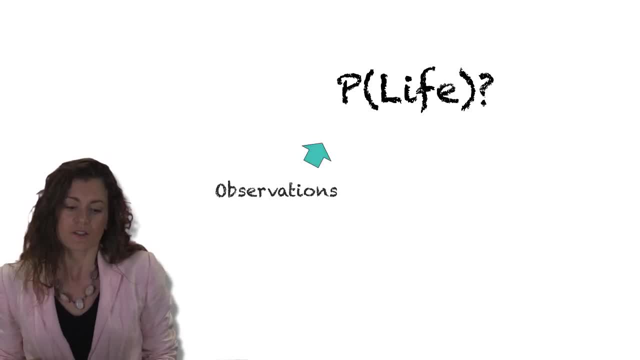 that as a planetary scale process And there's really two ways of constraining the likelihood of life emerging on a planet. We don't think that Jupiter is a living planet. Obviously, based on our observations of Jupiter, it could be that it might satisfy some definition of life. 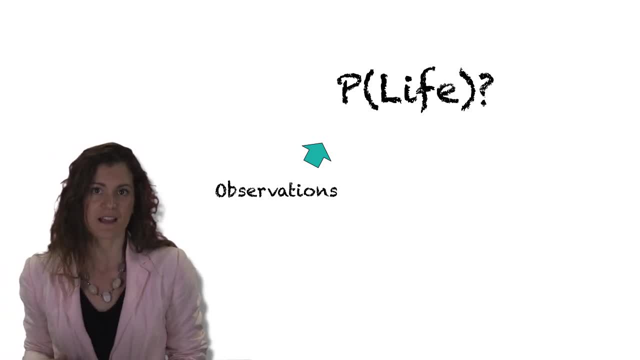 down the road if we actually come up with a theory for life and Jupiter satisfies that theory. But right now we don't think Jupiter is alive. So we need some observations of other living worlds to constrain the probability of life. Right now Earth is the only example we know. 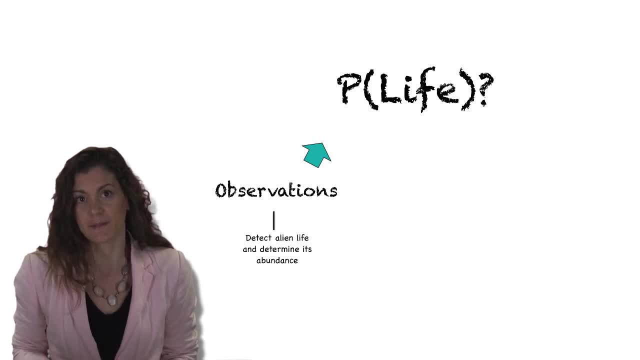 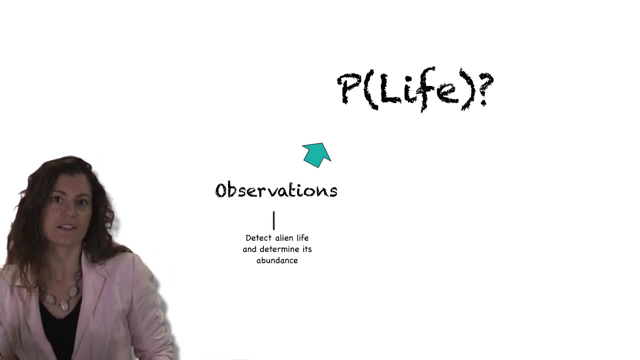 So to do that, we actually have to detect alien life and determine its abundance, And so this is the way usually people think about astrobiology: is actually looking at other worlds, trying to identify if there's aliens on those worlds, and then maybe we would actually be. 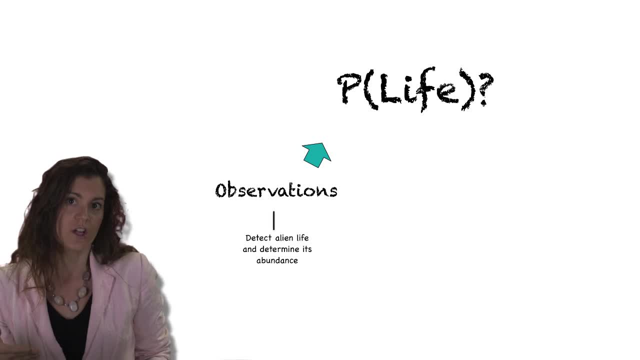 able to constrain the probability that a planet like Earth is going to emerge, life on its surface, and a planet like Jupiter is not. But we can also think about theory and experiment to constrain the probability for life And from this view the idea is really to try to uncover what are 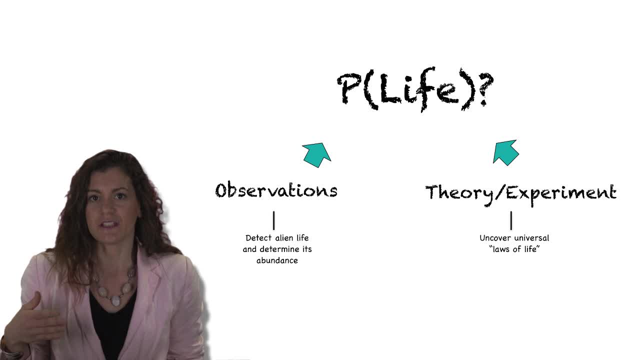 the universal principles of life that might actually allow us to build predictive models for the circumstances under which life should emerge. So we would have some a priori theory that would enable us to predict P-life, the probability of life emerging. And so, with the 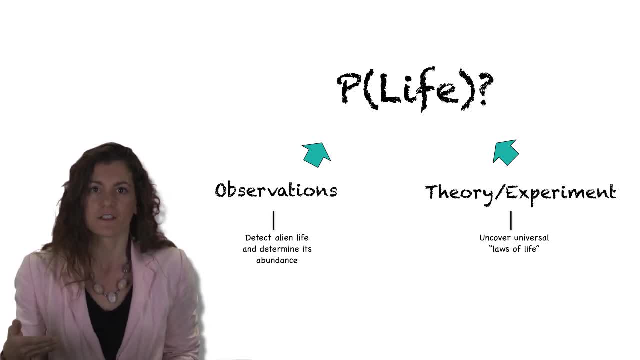 Earth example I gave. that theory should be able to account for the differences, that it's not just a non-equilibrium process on the surface of a planet, but in the case of formation of cities or forests or any of the kind of rich structure that we see on Earth, that's a product of biology. 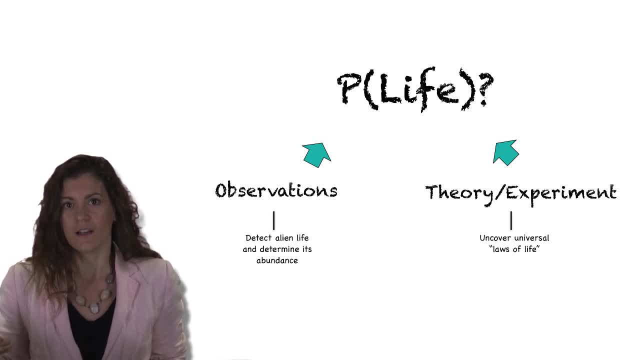 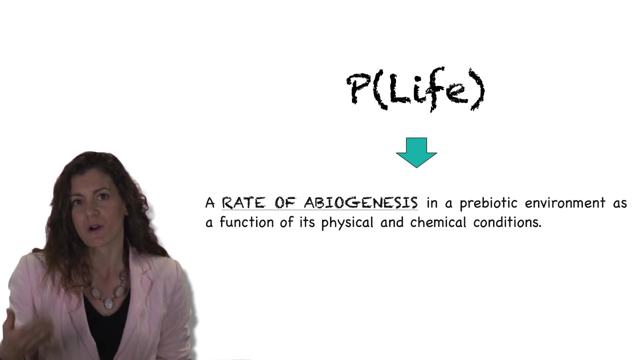 that the theory would be able to explain what those things are and be able to predict what kinds of other examples of life we might be able to see on other planets and their likelihood. But really what we're talking about- in order to constrain the probability of life- is not. 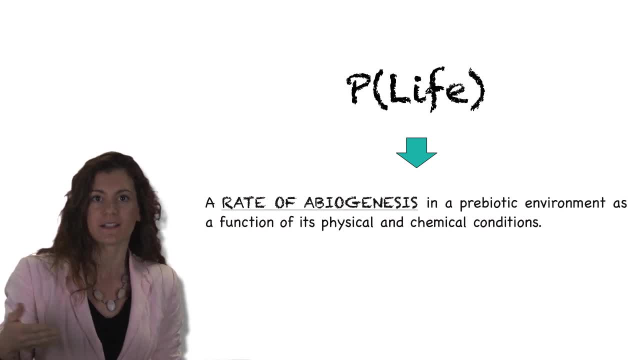 just to think about the probability of forests or cities on the surface of planets, as opposed to the probability of great red spots or other kinds of dissipative structures that aren't alive. What we really want is to understand what's the likelihood of life even emerging. 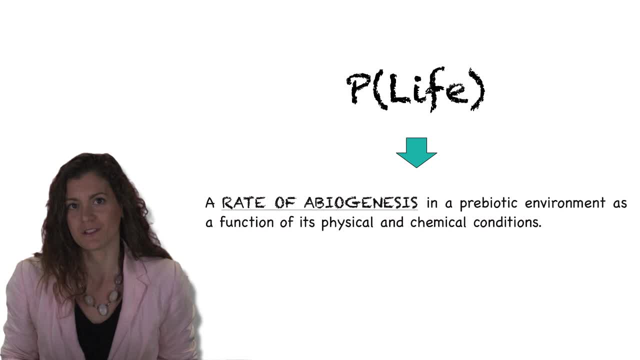 on that planet. So we really need to be able to solve the original life problem in order to do astrobiology effectively and constrain the likelihood of life in the universe. So that's what we're talking about: in order to constrain the probability of life even emerging. 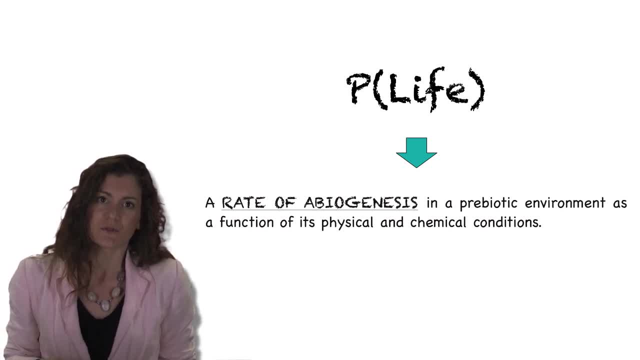 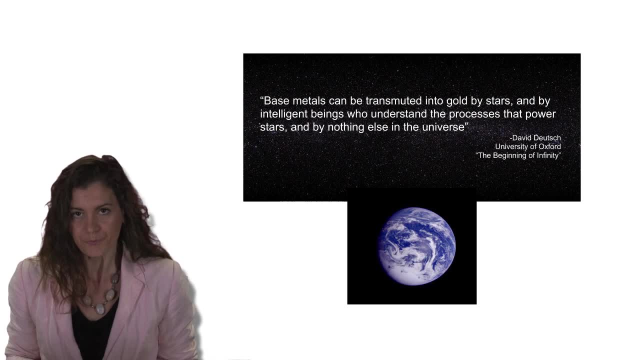 on that planet, And so, in order to do that, we have to come up with better theories for origins of life and be able to understand how life emerges, And so one of the ways I like to think about it is really that we're looking for new principles. 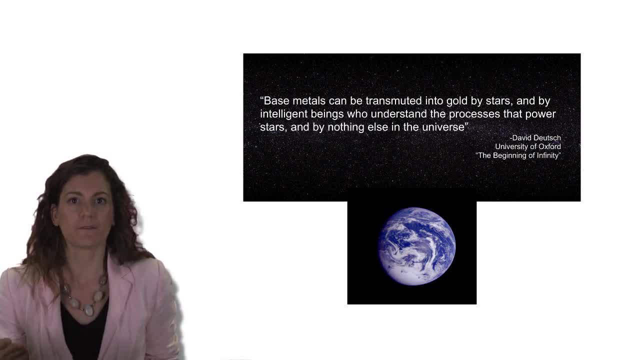 that would explain life, not just on Earth, but life on other planets, And I really love this quote from David Deutsch, which I think articulates very nicely the kind of processes that are happening on planets that we really need to be able to understand in order to 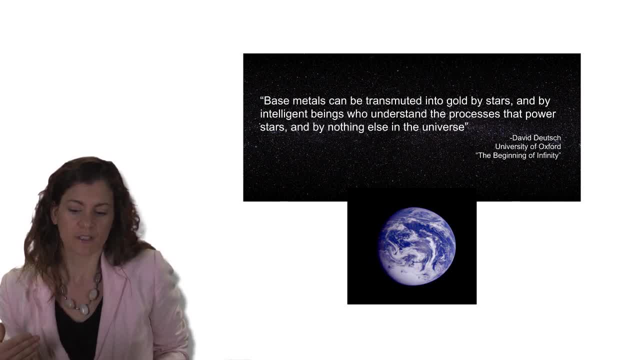 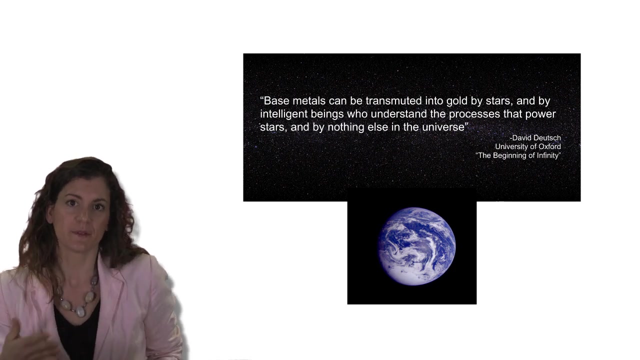 understand, And he says So. we have a physics that explains things like stars or the physics of Jupiter and why Jupiter has a great storm on the surface of the planet, the great red spot, But we don't have a physics that explains the evolution of a planet like our own, how life emerges.